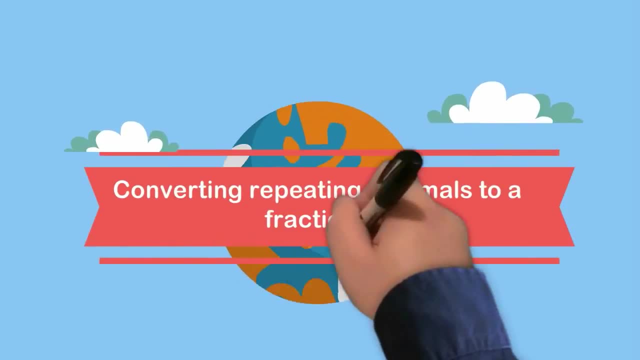 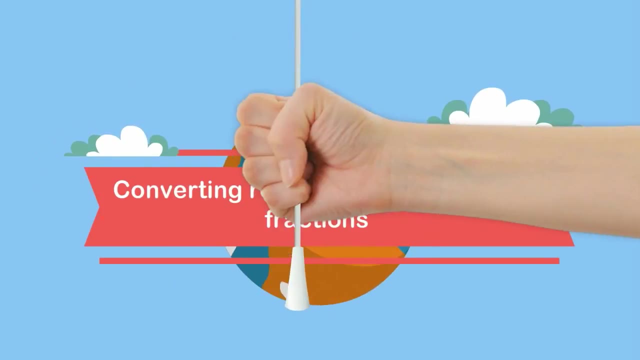 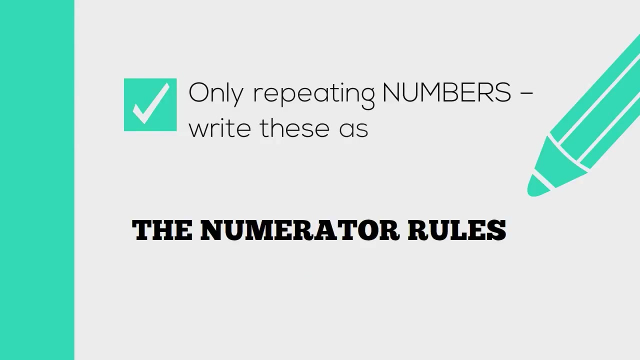 Welcome to MooMooMath and Science. In this video I would like to show an easy way for converting repeating decimals to a fraction. Lets go over a couple rules. First, the numerator rules. If you only have repeating numbers, write these as your numerator. 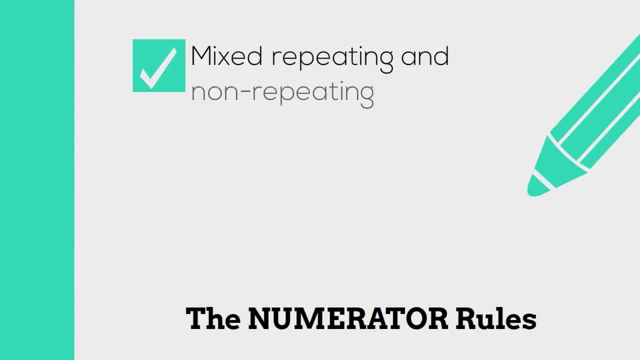 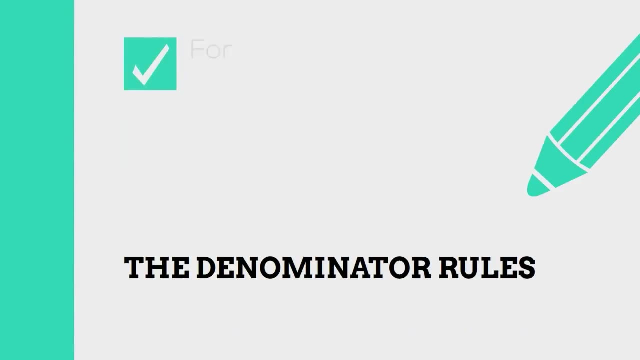 Or you may have mixed repeating and non-repeating numbers. If that is the case, write the non-repeating number, followed by the difference between the repeating and the non-repeating number. Now lets go over the denominator rules. For each non-repeating number, add a zero. For repeating numbers, add a nine. Lets work some examples and see if this makes sense. 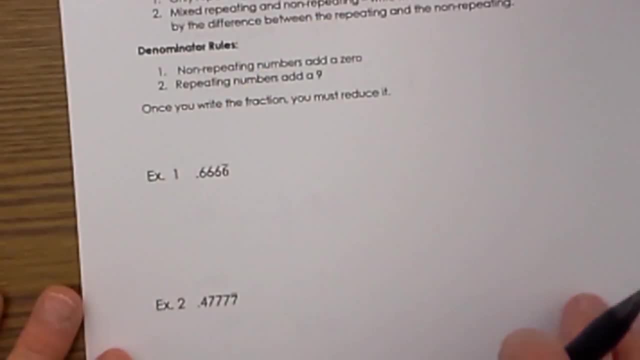 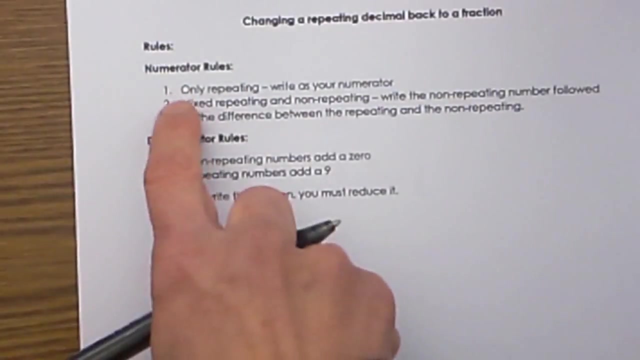 0.6666.. We are used to that and that is actually a pretty common one. We are going to look at the rules. This one has no non-repeating, It only has repeating. When we go to look at our numerator rules, we are going to use only repeating. 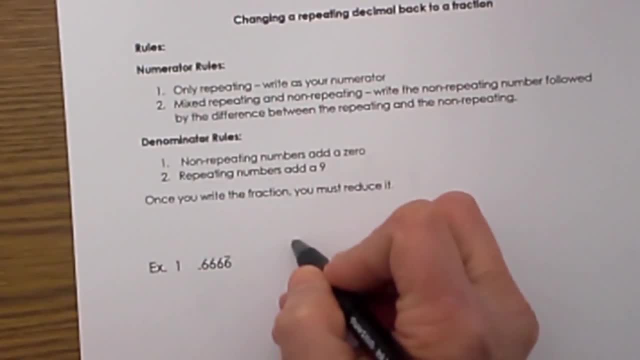 All we are going to do is use the six, because the six is the repeating number. That is the only number in my numerator For my denominator. I have repeating numbers, So I only have one repeating number and the six is repeating. So I am just going to add a nine, So six, ninths, and that is going to reduce now down by three. 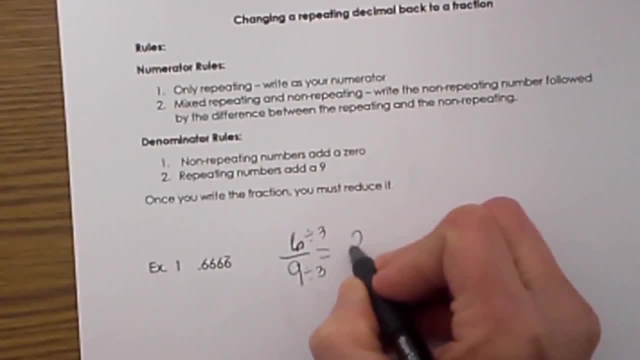 So I can divide this by three and divide this by three, So that is going to give me two thirds. If you want to check it on your calculator, you take two divided by three and you will see that it is 0.666 repeating. 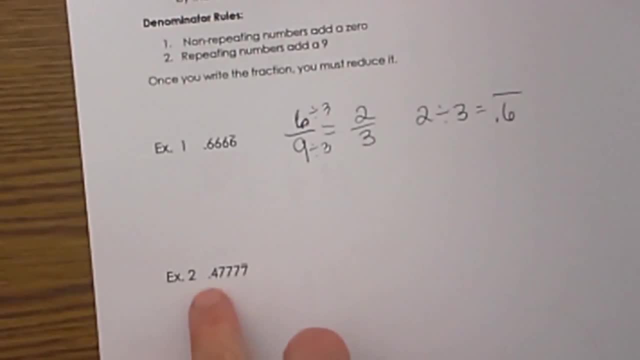 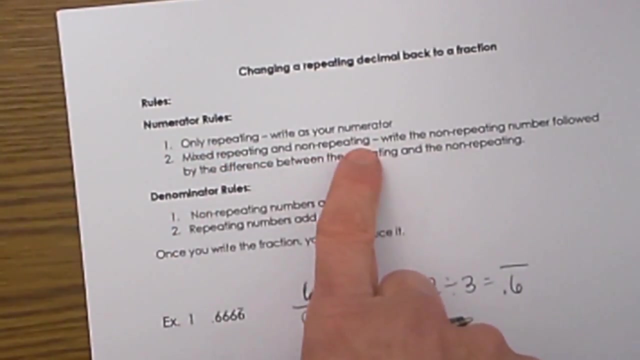 Now lets look at one that has some mixed repeating- 0.47777- and then seven repeats. So for the numerator I have a combination of things. I have mixed repeating and non-repeating. So write the non-repeating number, followed by the difference between the repeating and the non-repeating. 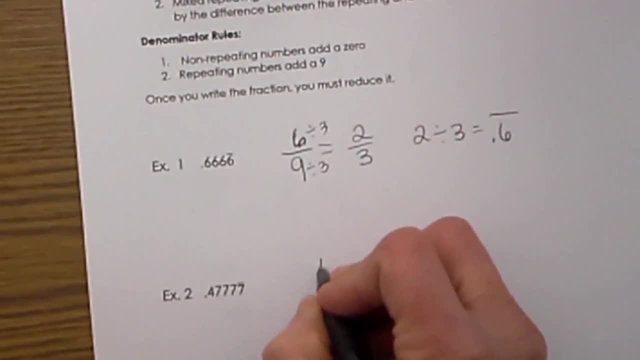 So my non-repeating number is four. so that is going to be the first digit in my numerator. Then I am going to follow it by the difference between the repeating and the non-repeating. Well, seven is my repeating, So I am going to take seven and I am going to subtract four, which is my non-repeating. 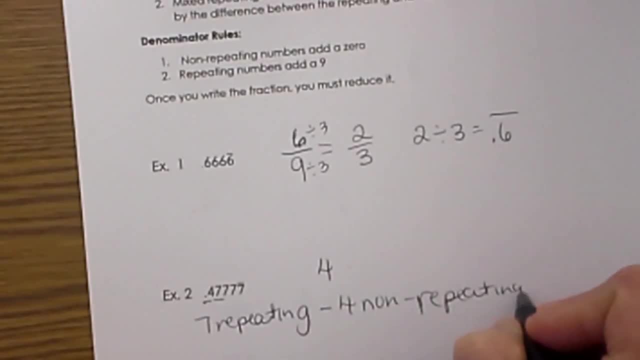 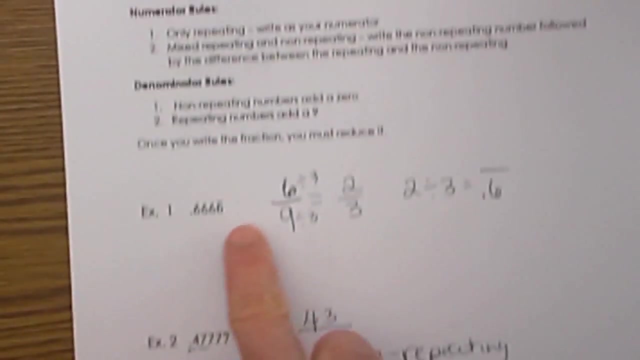 And that gives me the value of three. So I am just going to subtract seven and four. Now that is my numerator. Forty three is my numerator. Now to get my denominator. Seven is my repeating number. We said for denominators for repeating numbers, we are going to have a nine. 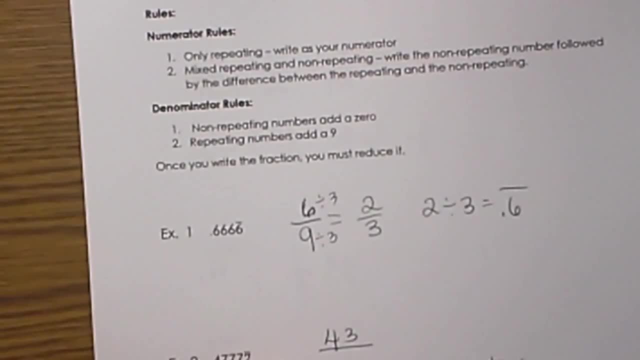 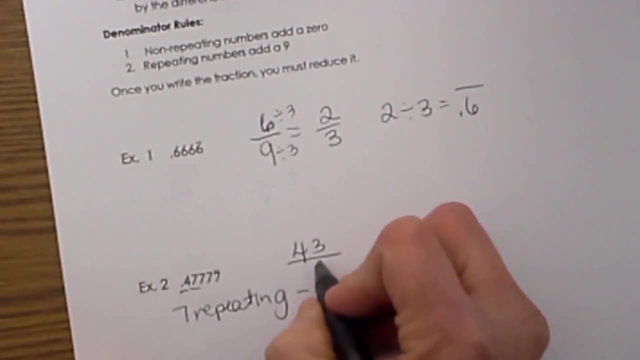 So I have one number I am repeating, which is the seven, And then my non-repeating number. I am going to have a zero, So I am going to have one nine and one zero. The zeros always go at the back, So it is going to be forty three over ninety. 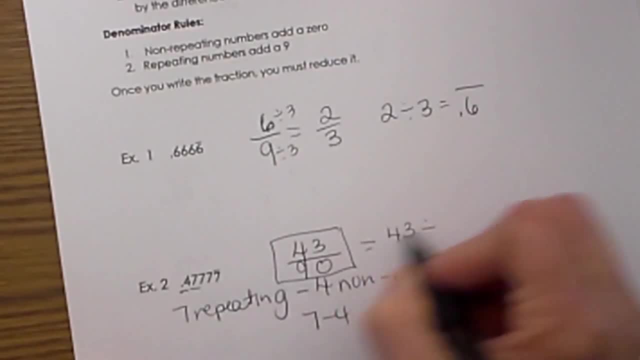 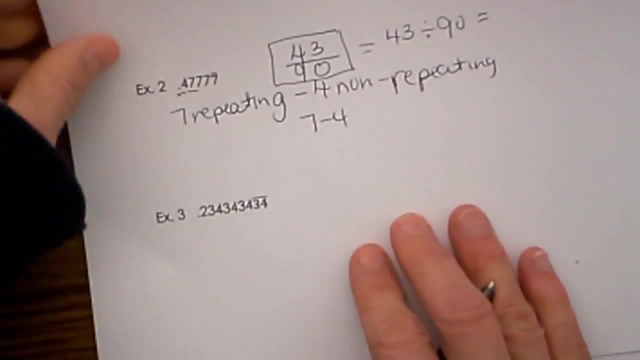 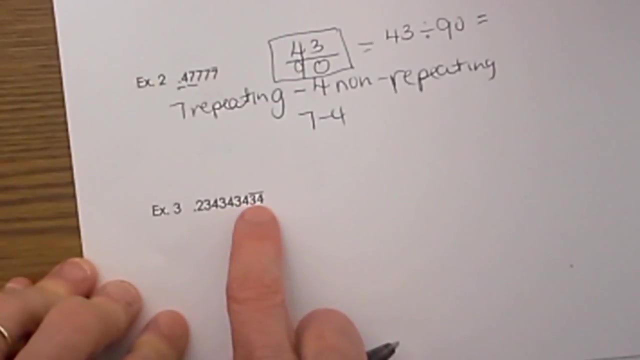 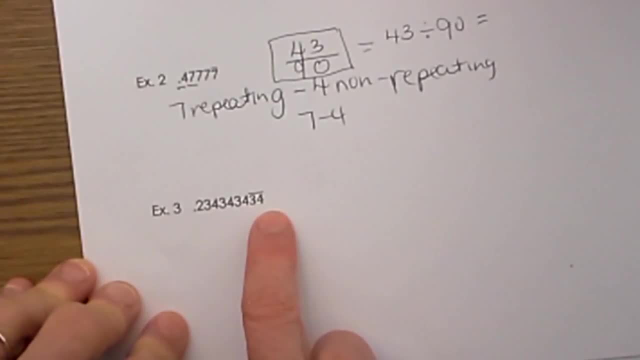 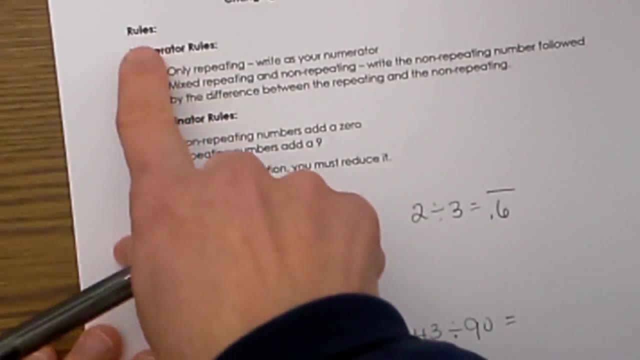 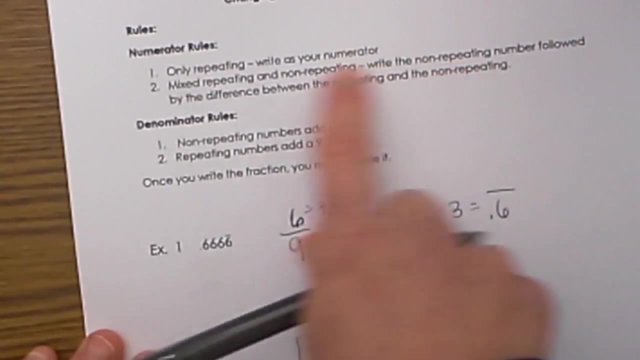 So thirty four is my repeating. number Two is my non-repeating. So let's go back up and look at our rules. So we have to look at the second numerator rule, repeating and non-repeating. We have them mixed, So write the non-repeating number first, followed by the difference. 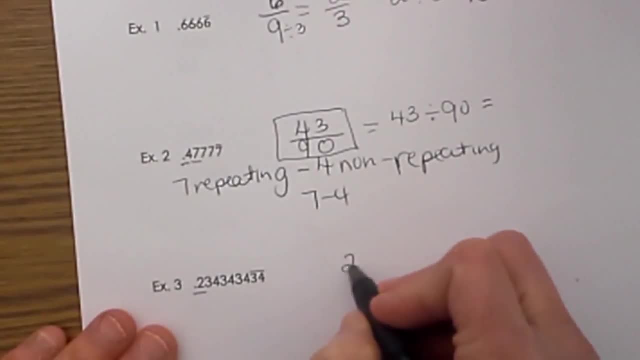 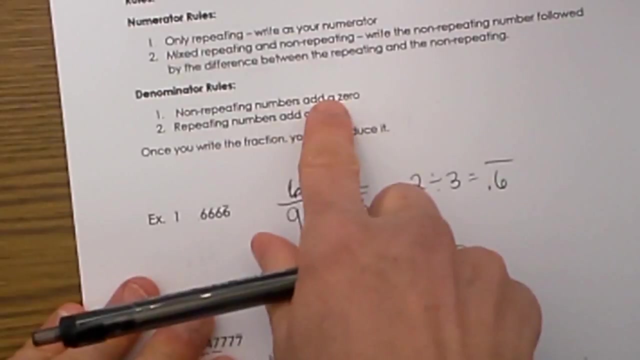 So my non-repeating number is two. The difference between thirty four and two is thirty two, So two hundred and thirty two is my numerator, Now my denominator. For every non-repeating number I have a zero, And for every repeating digit I have a nine. 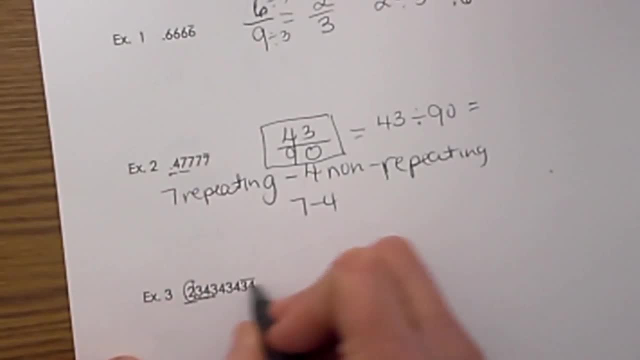 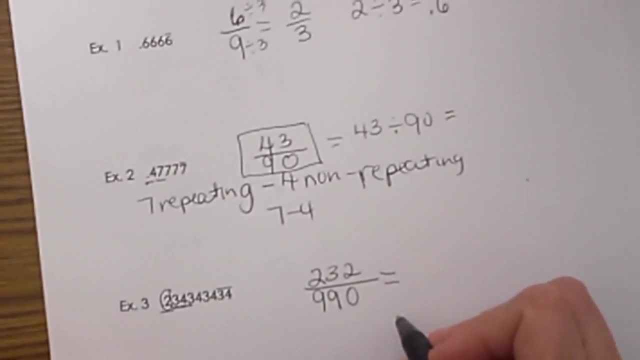 I have two digits, A three and a four, that keep repeating, So that is two nines, And then my non-repeating two. So there, two hundred and thirty two over nine ninety is this decimal, And I can reduce that. Let's see.